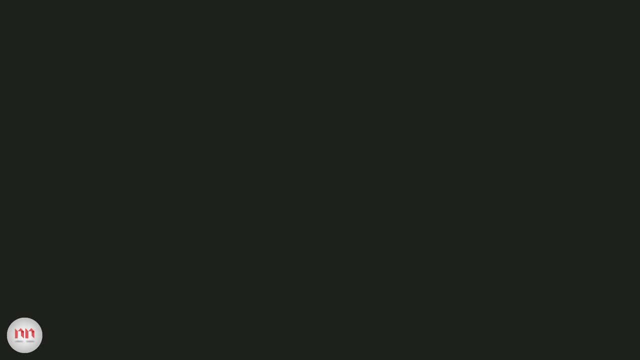 our friend Jack, who lives in a hypothetical town. There exist only three kinds of weather in that country: cloudy and sunny. On any given day, only one of them will occur, And the weather tomorrow depends only on today's weather. Yes, we can model this as a simple Markov chain. Let me add the state. 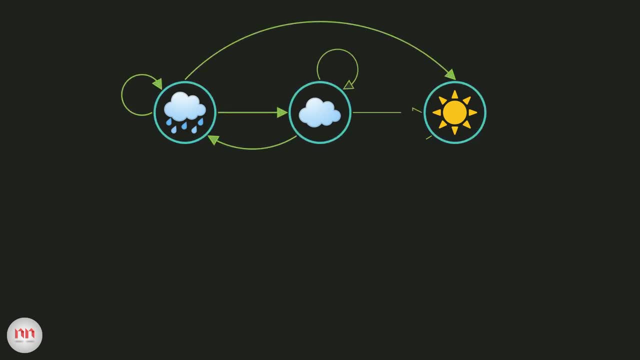 transitions, And here are the transition probabilities. Also assume that on any given day Jack can have one of the. also assume that on any given day jack can have one of the. also assume that on any given day jack can have one of the. 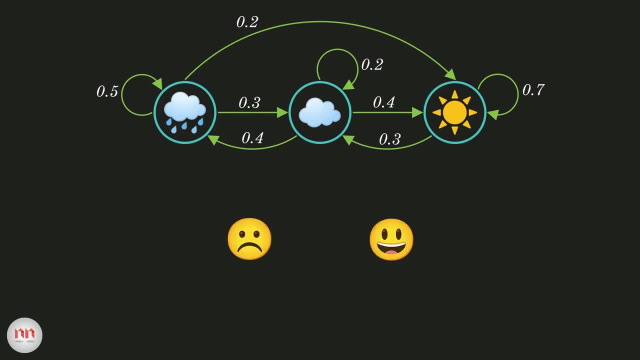 two following moods: sad or happy. moreover, his mood depends on the weather of that particular day. i'm gonna represent it with red arrows. here are the corresponding probabilities. so, according to our diagram, there's a 90 chance that jack is sad, given that it's a rainy day. 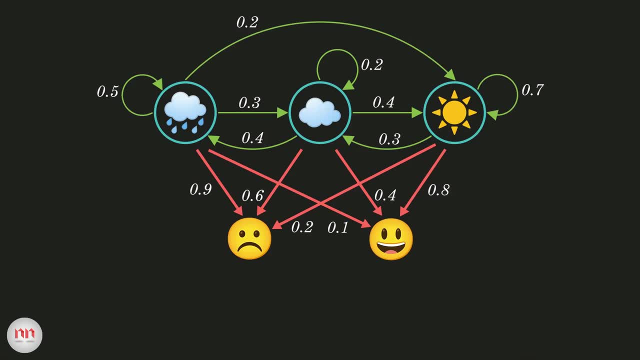 hopefully it's clear to you too. okay, so now our problem is: we don't live in jack's town, so we can't possibly know what's the weather on a particular day. however, we can contact jack over the internet and get to know his mood. so the states of the markov chain are unknown or hidden. 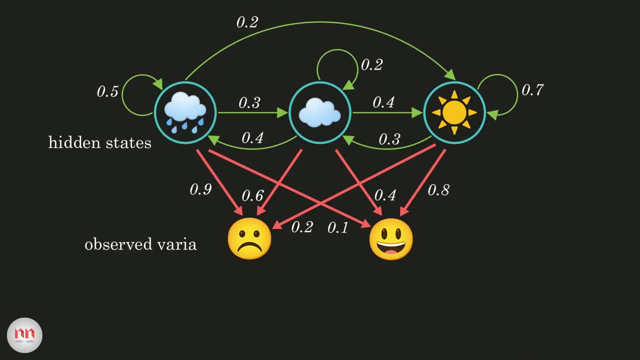 from us, but we can observe some variables that are dependent on the states, and this, my friend, is called a hidden markov model. in other words, a hidden markov model consists of an ordinary markov chain and a set of observed variables. please note that jack's mood. that is the observed 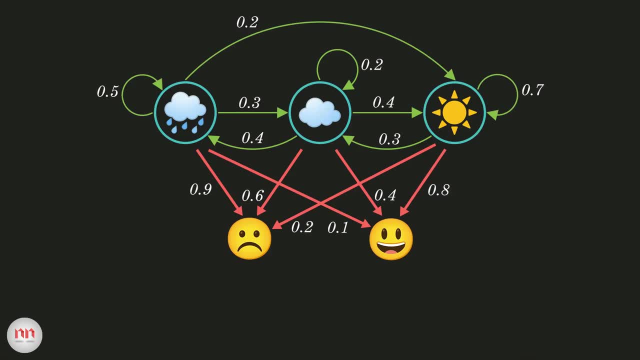 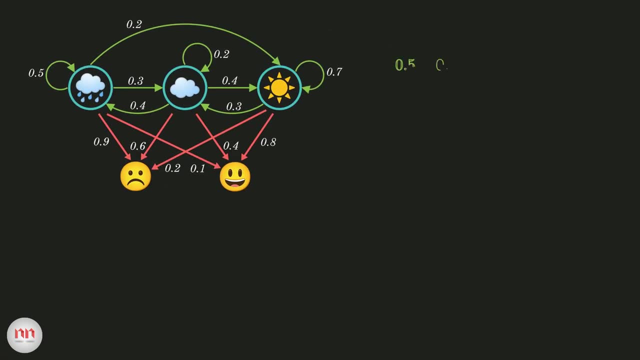 variable depends only on today's weather, not on the previous day's mood. to make things more clear, i'm gonna write the probabilities into a matrix. you are already familiar with the green matrix, that is the transition matrix, and the red one captures the probabilities corresponding to the observed variables. 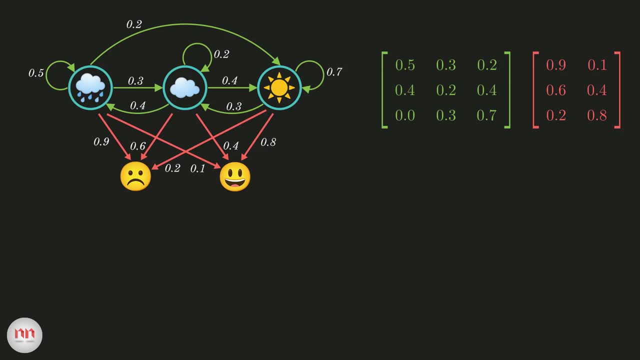 which is also known as the emission matrix. let me add the indices to make it more interpretable. this is the correct time to pause and convince yourself that you have understood everything so far. okay, let's consider a particular scenario. we will look at three consecutive days. suppose on the first day it was sunny and jack was happy. next day was cloudy and 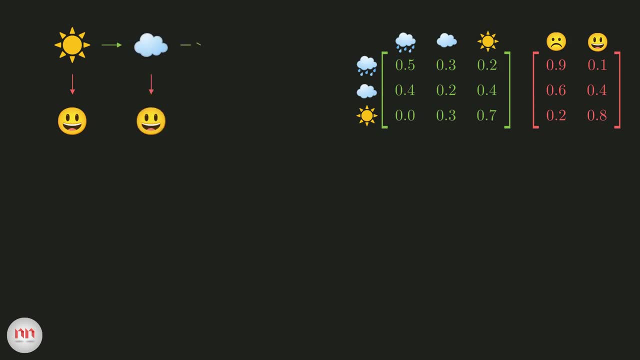 jack was happy, and on the third day it was sunny again, but jack was sad. well, i know that we can't observe the hidden states, but just assume that this scenario happened. trust me, analyzing this will help us a lot. okay, the question i want to ask here is: what is the probability of this scenario? 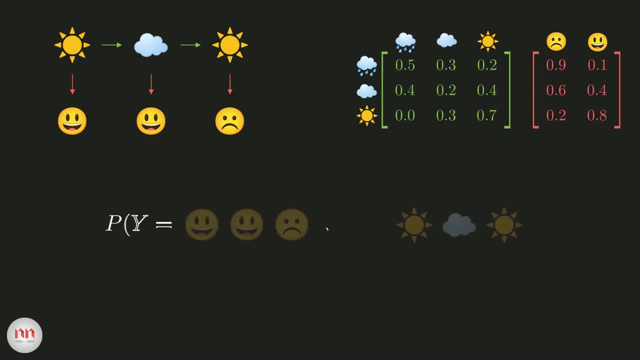 occurring. more precisely, what is the joint probability of the observed mood sequence and the weather sequence? pause here. if you'd like to try by using the markov property, we can compute this as a product of six terms. first the probability of a sunny day, then the probability of happy mood given a sunny. 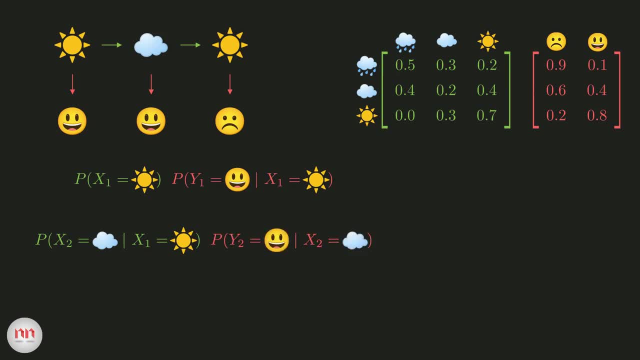 day, then the transition probability from sunny to cloudy and so on. but how we got these six terms? please bear with me till the end to understand the underlying mathematics. we can fill the red terms from the emission matrix and the green ones from the transition matrix. but what about the first term? how can we find the probability of the first state? 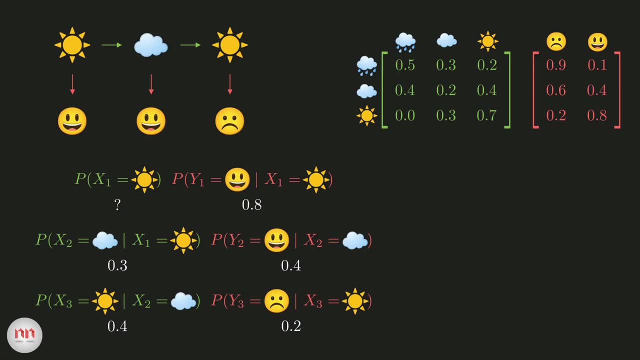 yes, we need the stationary distribution of the markov chain. for this purpose, you can use the normalized left eigenvectors or repeated matrix multiplication to compute the stationary distribution. i have explained both of them in my previous videos. so, as you can see, the sunny state has the probability of 0.509. now we can compute the. 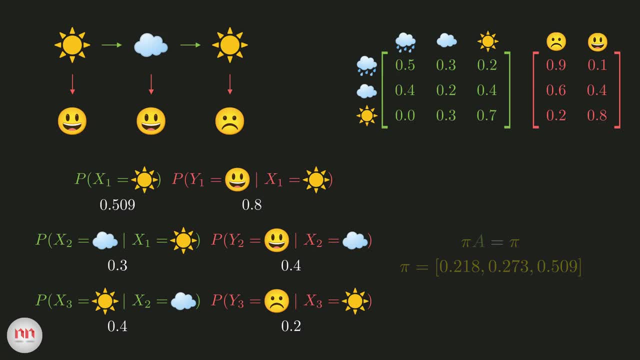 product and the answer turns out to be 0.00391. okay, let me hide the states now. so we only have a sequence of the observed variable here. i'm going to ask a more interesting question: what is the most likely weather sequence for this given mood sequence? hmm, there are many. 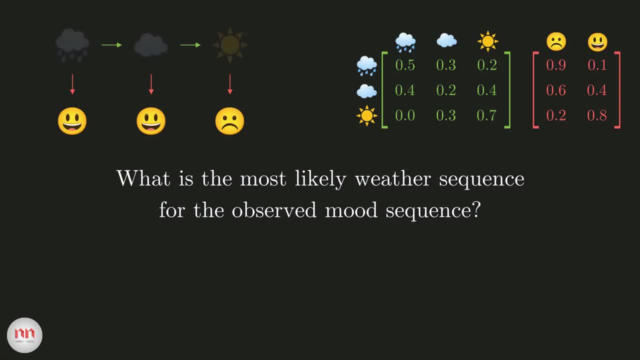 possible permutations right. we can have rainy, cloudy, sunny, cloudy, rainy, sunny, rainy, cloudy, rainy, and so on. to find the most likely sequence, we need to compute the probability corresponding to each of them and find the one with the maximum probability. we can calculate the probability just like we did in the last case. i wrote a python script to do the computations. 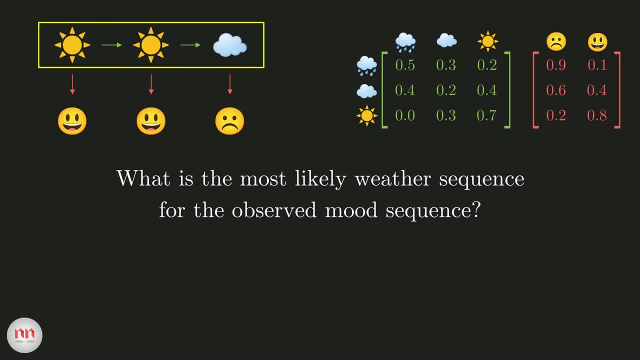 and found that this way, the sequence maximizes the joint probability and the probability is 0.04105, are still watching this. i believe you would also like to know the formal mathematics behind this, so get ready for some symbols instead of emojis. i will represent the hidden states of our markov chain. 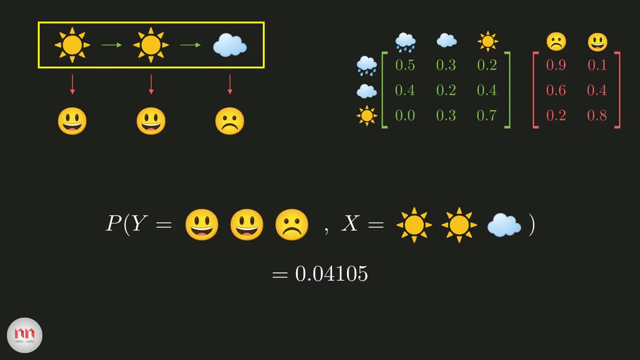 by x and the observed variable by y. we can rewrite our problem like this: this simply means find that particular sequence of x for which the probability of x given y is maximum. please note that in a hidden markov model we observe the sequence of y. that's why i have written x given y. now, if you notice carefully, you will see there's no direct 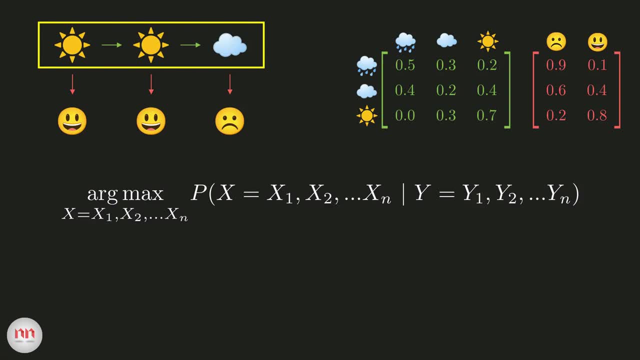 way to find this probability. here comes the base theorem. by the way, i have a video explaining base theorem. you can watch that if you want. so by using base theorem, we can rewrite this as the probability of y given x, the probability of y given x by a random variable. 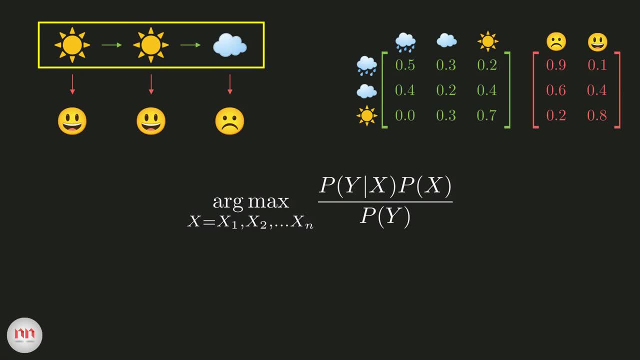 we can write the probability of y times the probability of x upon the probability of y. for all practical purposes, we can neglect the denominator, and the numerator is just the joint probability distribution of x and y. now we are going to further simplify this. let's take the 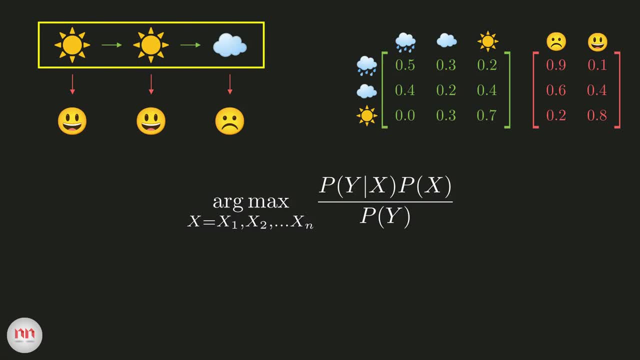 first part, the probability of y given x. according to our assumption, yi depends only on x. i probability of Y given X as a product. We can fill all these terms from our RAID matrix. For the second term, probability of X, we must use the Markov property that says Xi depends only on Xi-1.. So we can. 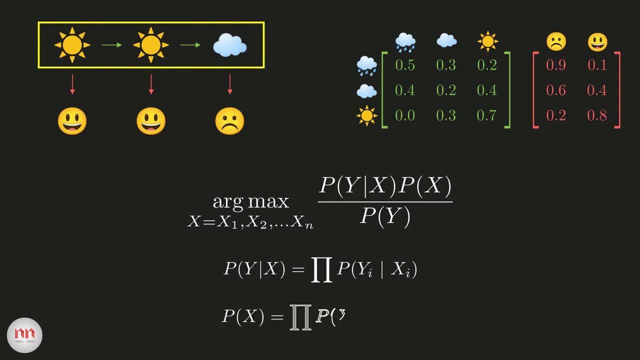 convert Px into this product. Now there's one subtlety involved: For X0, we must use the stationary distribution vector, as I already showed you earlier. Okay, so now replace these things into the above expression and we have got the thing that we want to maximize. You can clearly see that this expression is just 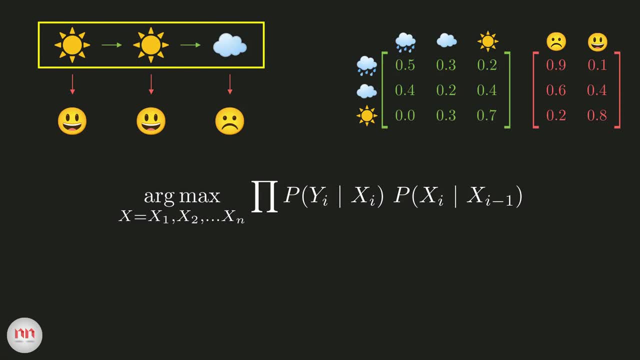 a product of two n terms. I hope now you fully understand the origin of those terms In the example that I computed earlier. Isn't it super elegant? Well, I guess it is. I know it's not the easiest thing, So don't worry if you didn't get everything. 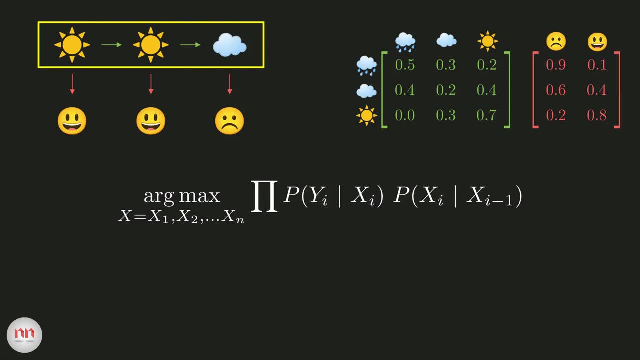 at once. You can always replay the video to remove your confusions. So that was all for this video. guys, Do comment below your thoughts and suggestions, and subscription will be a major help to me. Goodbye, guys, stay safe and thanks for watching. Subtitles by the Amaraorg community. 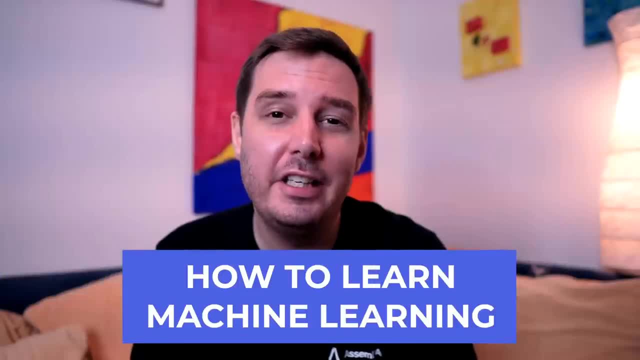 Hi everyone, I'm Patrick and in this video I show you how I would learn machine learning, if I could start over For context. I'm a machine learning developer advocate at Assembly AI and before that I worked several years as software developer and ML engineer. 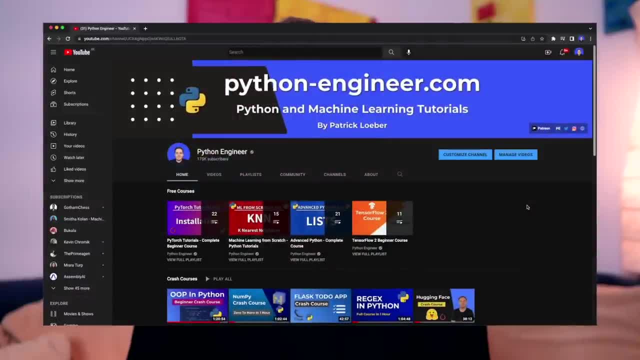 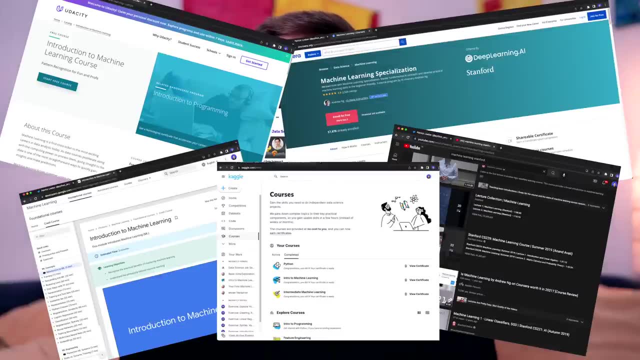 and I also teach Python and machine learning on my own YouTube channel, so I would say I'm pretty experienced in the field, But I know that the available courses out there can be overwhelming for beginners, so I hope to give you some guidance with this video.